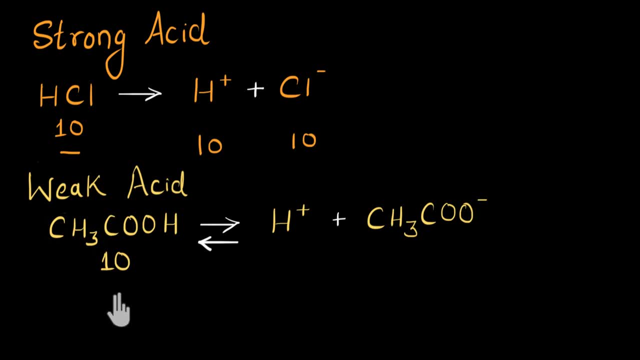 of acids in our solution and at the same time we have to keep our sources intact. So for existing acid molecules still in the solution, Let's say maybe eight molecules are still in the solution And only two molecules have dissociated to give us H plus and acetate ion. 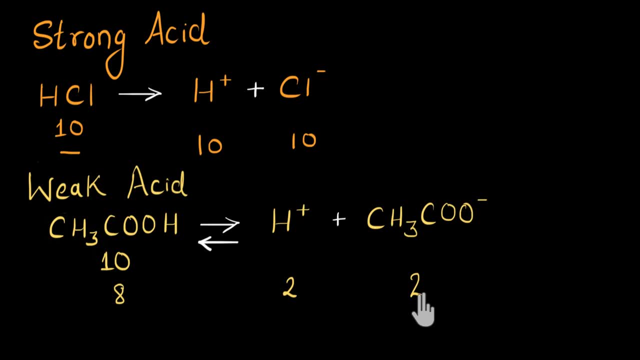 The rest of the molecules would have dissociated, but their ions would have combined back to give us the acid molecule. okay, So this is the difference between strong acid and weak acid. See strong acids. they undergo complete dissociation, meaning all the molecules of the acid will dissociate. 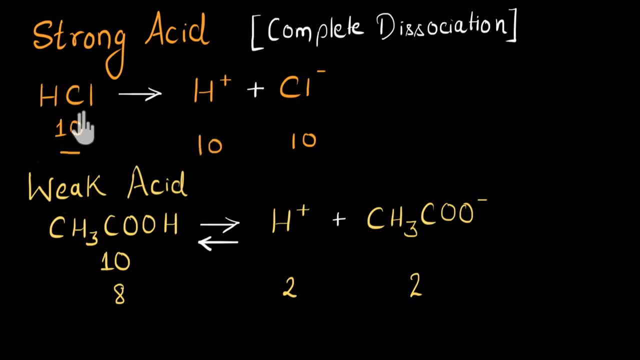 to give us H plus ion And no molecules of the acid will remain back in the solution, Whereas weak acids, they only undergo partial dissociation, meaning not all molecules. In fact, only few molecules of the acid will dissociate to give us H plus ion. 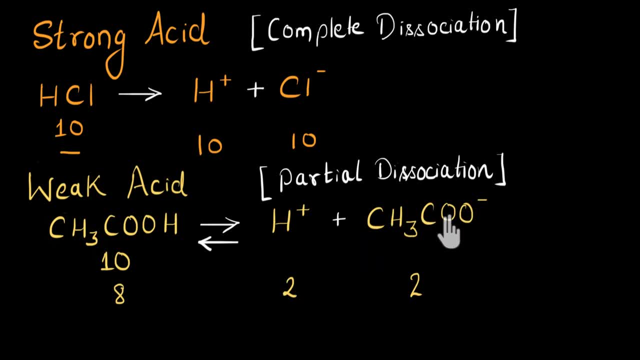 And that is happening because the negative ion that gets formed is very unstable. It combines back with the H plus to give back the acid. Okay, now this means that if I take equal amount of strong acid, this will give me a lot more H plus ions. 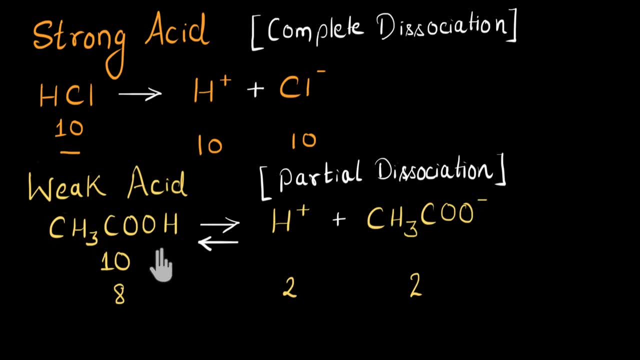 than the equal amount of strong acid. In fact, weak acids, they give us very little amount of H plus ions And that's why they are less harmful or less dangerous to a human body And strong acids, since they give a lot of H plus ion. 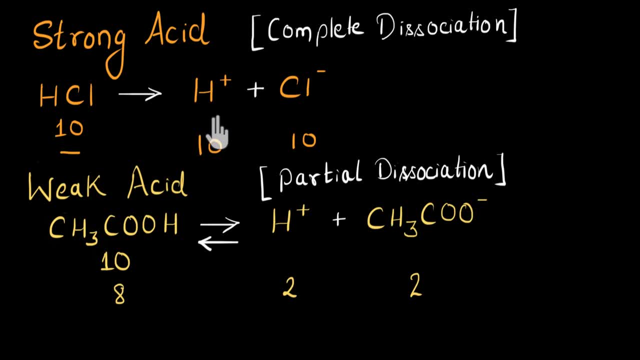 they could be very dangerous to human body Because, see human body, it tries to maintain the acidity of the body or the concentration of H plus ions in the body, And whenever it comes in contact with even small amount of strong acid, it could increase the concentration of H plus ions. 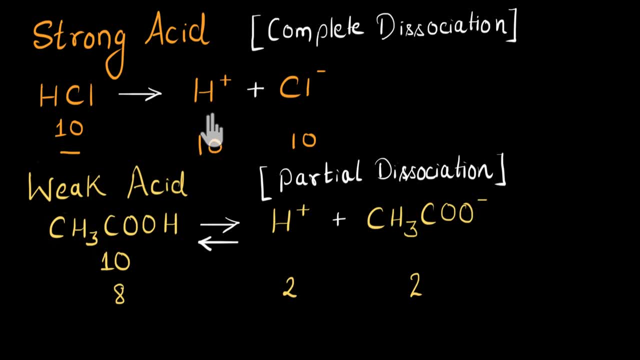 And therefore it can harm the human body. That's why we suggest, you know, be very careful around strong acids. Later on we will study how to dilute these strong acids and use them safely, But for now, let's look at some examples. 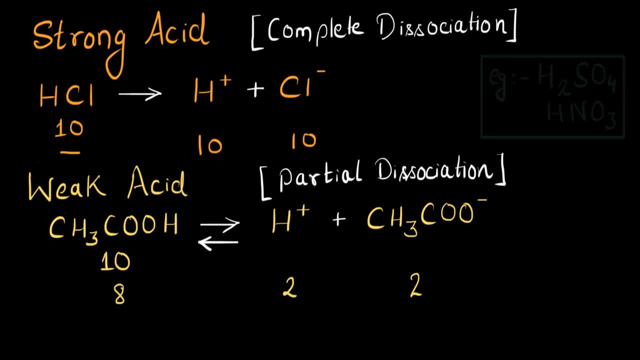 of strong acid and weak acids. So strong acid, apart from HCl, is H2SO4,, HNO3, and other acids. See all of these acids. they completely dissociate, meaning you would not find their molecules present in the solution.